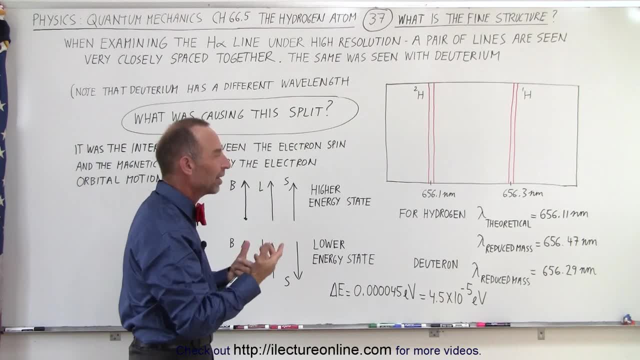 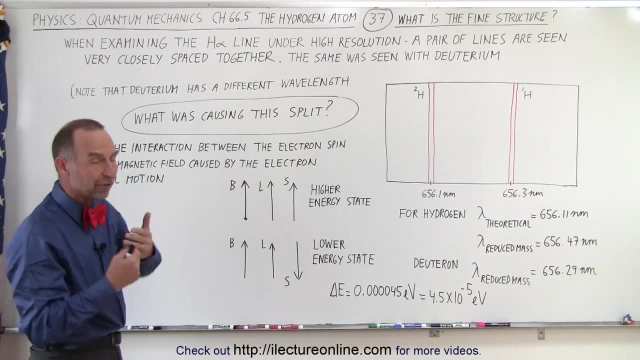 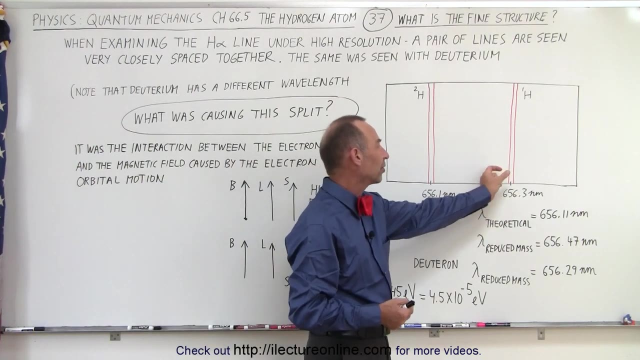 again we'll see the very closely spaced two lines representing the H-alpha jump, the first Balmer series jump, where the electron jumps from the third to the second energy, giving us a visible photon of red light. The wavelength is about 656 nanometers, but you can see the very 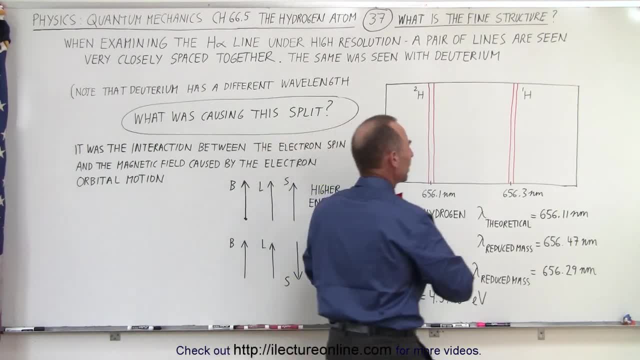 narrow spacing between the two. Matter of fact, the spacing between the two is somewhere in the order of zero. So if we look at the H-alpha line, we can see that the H-alpha line is about 656 nanometers, but you can see the very narrow spacing between the two. Matter of fact, the 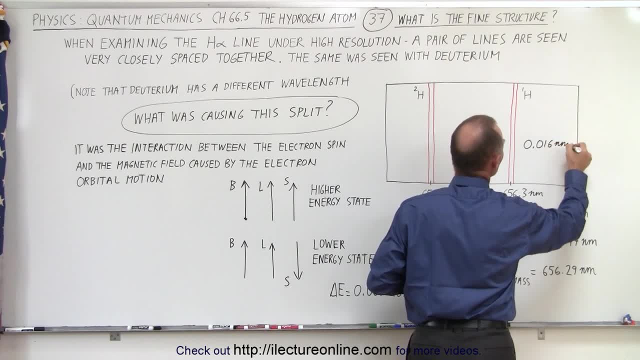 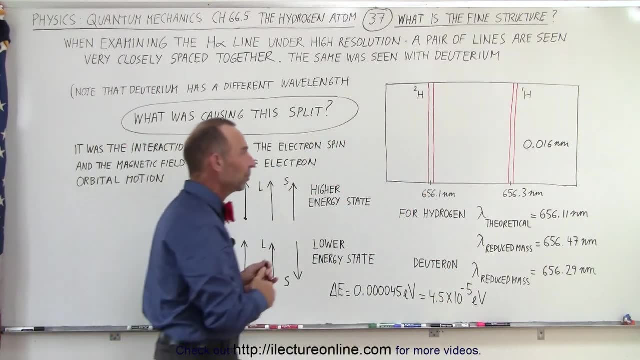 H-alpha line is about 656 nanometers, but you can see that the H-alpha line is about 656 nanometers, but you can see that the H-alpha line is about 0.016 nanometers. So you can see that they're very, very closely spaced together. Now there's a slight difference between the H-alpha 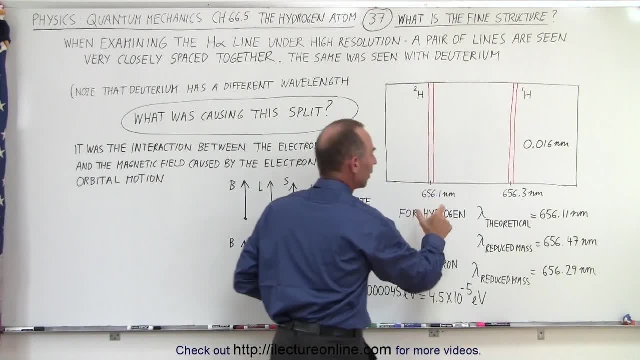 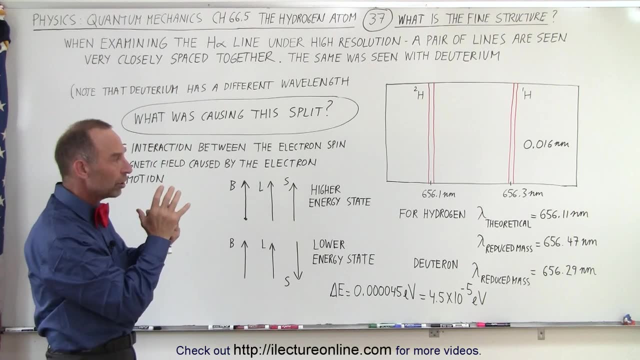 line that we get from a deuteron versus a single hydrogen atom. The difference- it's only 0.2 nanometers- is because the deuteron has a neutron in its nucleus, which causes the reduced mass to be a little bit different, And we'll talk about the reduced mass affecting the wavelengths that we get. 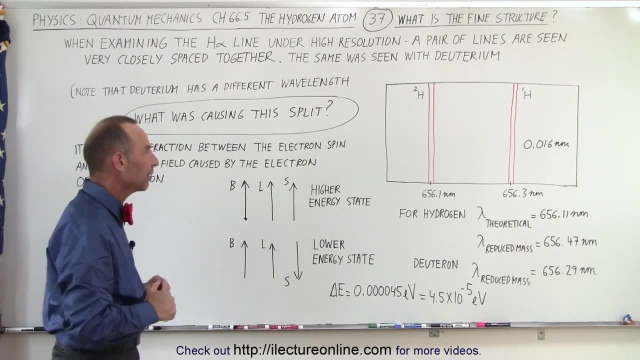 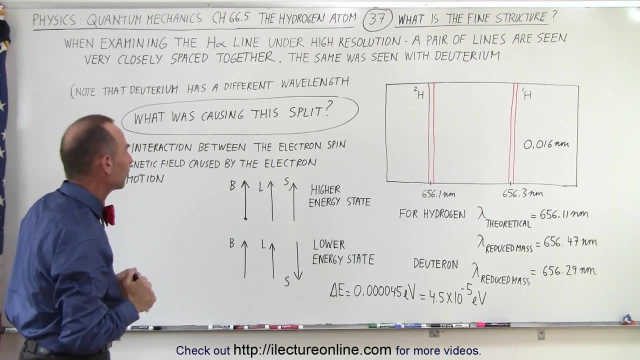 from the deuteron, And we'll talk about the reduced mass affecting the wavelengths that we get from the electron jumps, and we'll talk about that in a different video. So what is causing this split? Why do we see those two very fine lines very closely spaced together? Well, it turns out. 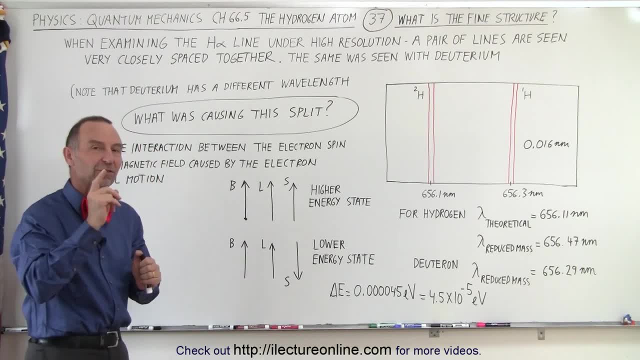 it's actually caused by the interaction between the spin of the electron. All small particles like that have intrinsically a spin property. It's kind of like something turning on its own axis, although it's not quite that for the electron, but it has the same kind of property as spinning on. its own axis And it's kind of like something turning on its own axis, although it's not quite that for the electron, And it's kind of like something turning on its own axis, although it's not quite that for the electron, And it's kind of like something turning on its own axis, although it's not quite. 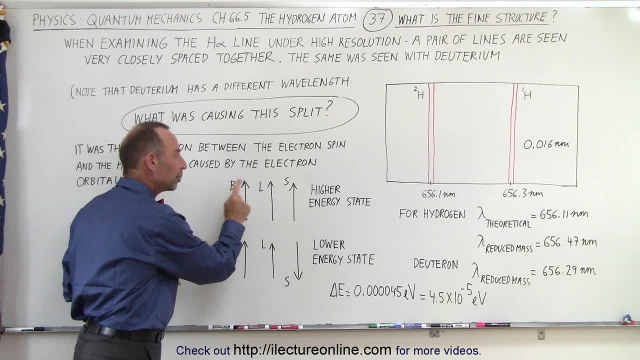 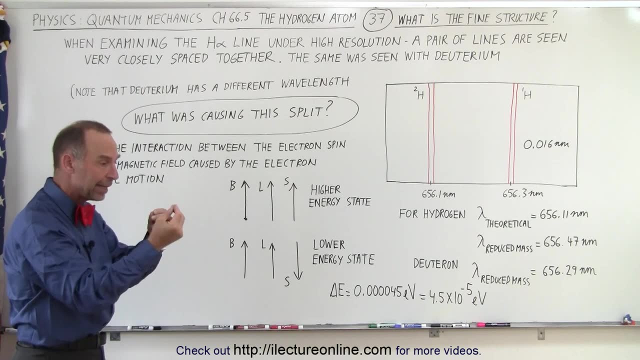 Alors, the spin acts on the DAV. Possibly the annulment actually causes that discrimination, because the spin reacts by the orbital motion of the electron And what we'll see is that spin interacts with the magnetic field produced by the orbital motion of the deuteron. Essentially, the electron zips on the 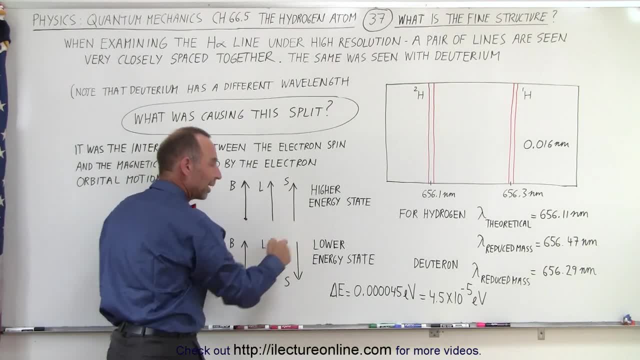 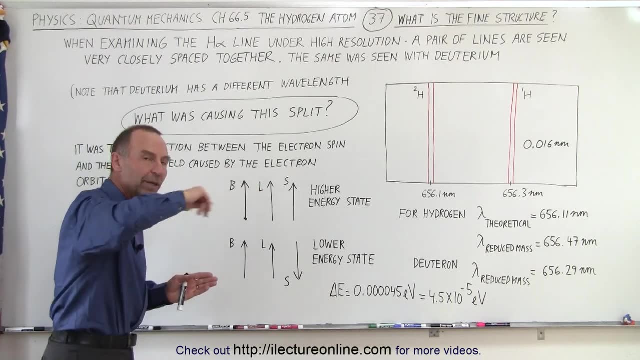 that the spin direction can either be spin up or spin down. now it's not exactly the way we've shown here, but essentially that's what it is. the electron can spin in one direction or it can flip over and spin in the other direction again. that's quantum mechanically, and then you can see the 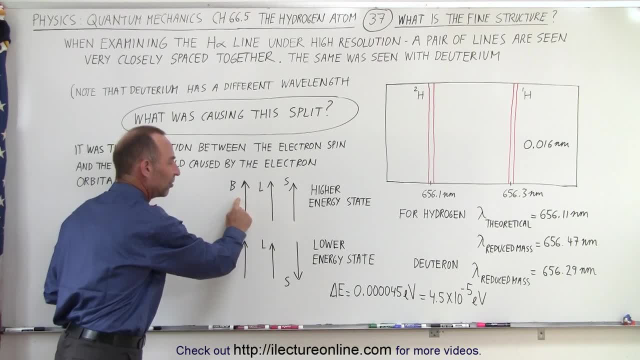 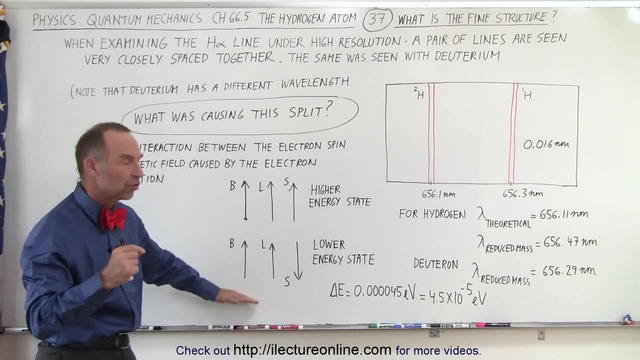 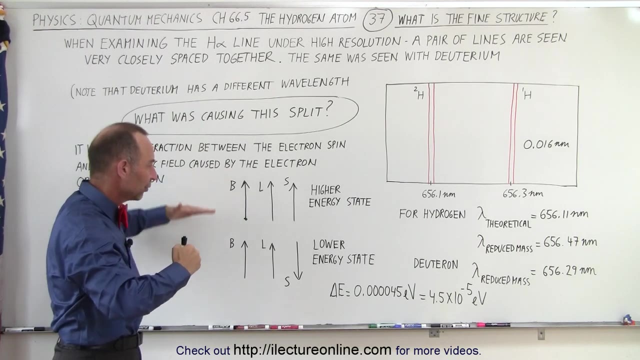 interaction would be different: between the spin direction and magnetic field in this case, and the spin direction, magnetic field in this case. this ends up being a higher energy state. this ends up being a lower energy state. so, depending upon from which point, from which interaction, the electron jumps from one level to another, if it jumps from a spin up condition versus spin down condition, 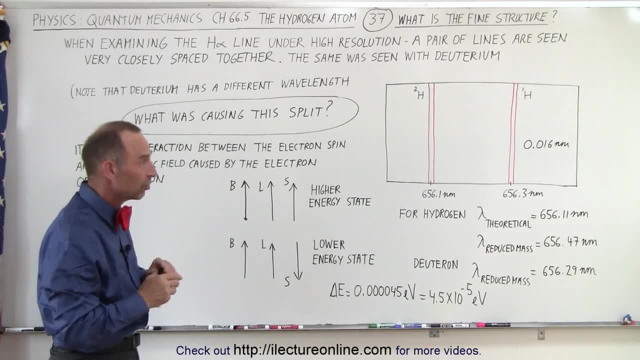 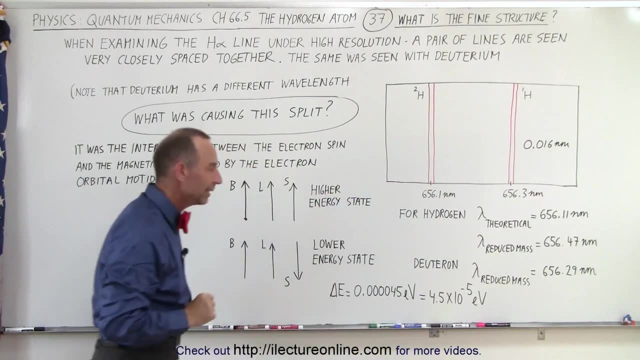 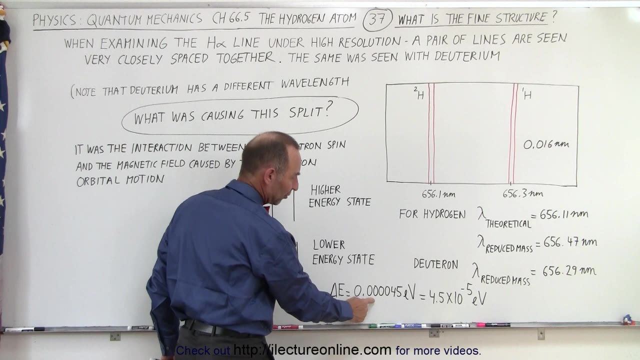 there's going to be a slight difference in the energy transition during that transition, which causes slight difference in the wavelength of the photon that's generated with a very small difference in the wavelength. now the energy difference between those two lines represents a very small energy of 0.05. 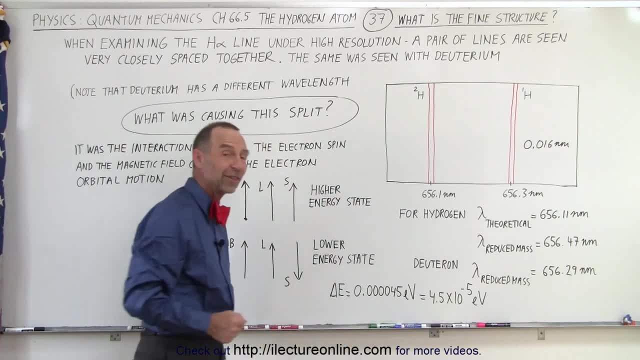 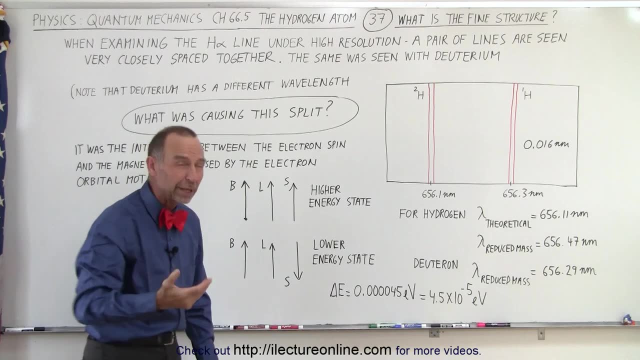 zero, zero, zero, zero. four or five electron volts, four point five times center, minus electron volts, and knowing that the energy of a h alpha line is typically in the order of about 1.8, 1.9 electron volts, you can see that's just a very tiny fraction and therefore a very small difference. but 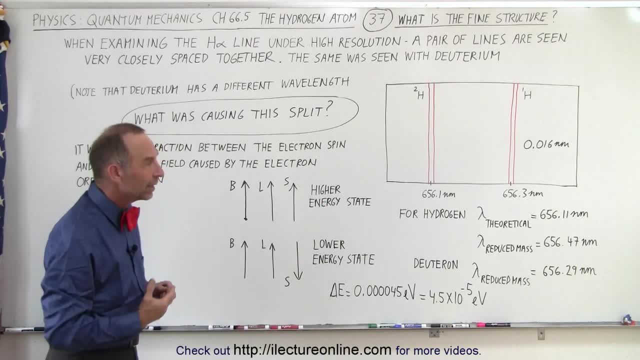 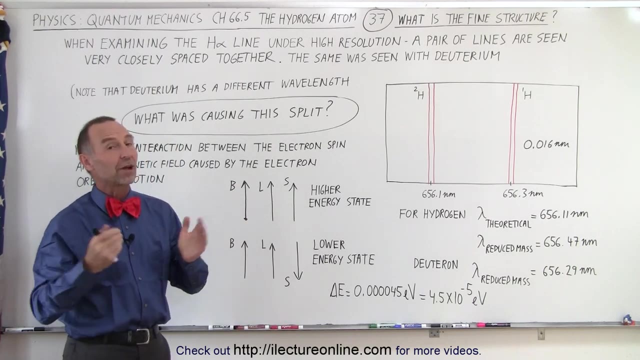 nevertheless it is there. they had to figure out why that line, that double line, was there. it's called the doublet and of course they found by looking at the interaction between the spin and the orbital motion, the interaction between the spin and the orbital motion, the interaction between the magnetic field of orbital motion and the spin direction of electron.